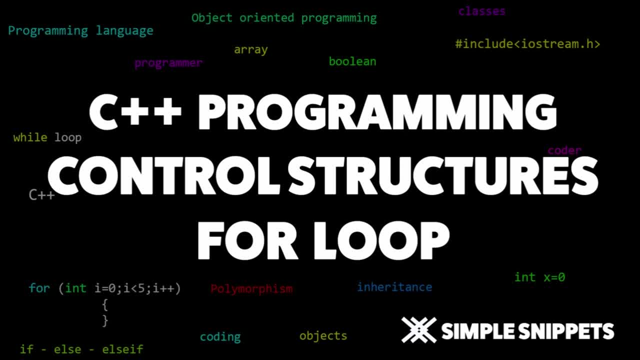 about conditional control structures, that is, if-else structure and switch case. So if you have missed that, you can check it out Now. this video tutorial is based on a looping control structure and specifically we are going to be discussing about for loop. 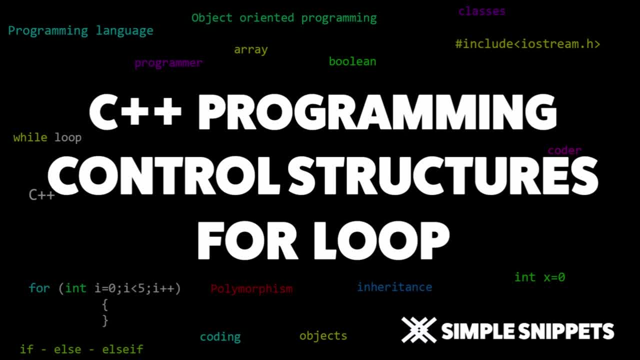 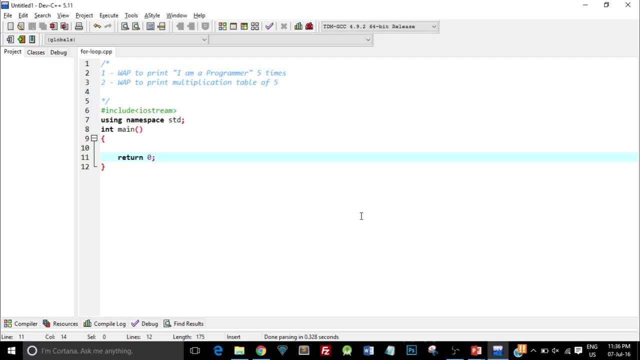 and we will see two different programs. With that being said, let's start with the programming part, because that is the best way you can understand this for loop structure. Okay, so, as you can see on the screen, I have opened my Dave C++ IDE and I have written the basic. 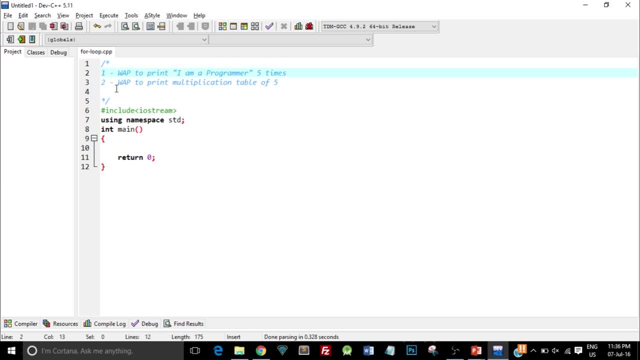 structure of a C++ program, and here on top you can see the two questions that I have written down. So the first one is: write a program to perform print- I am a program of five times- And the second question is: write a program to print. 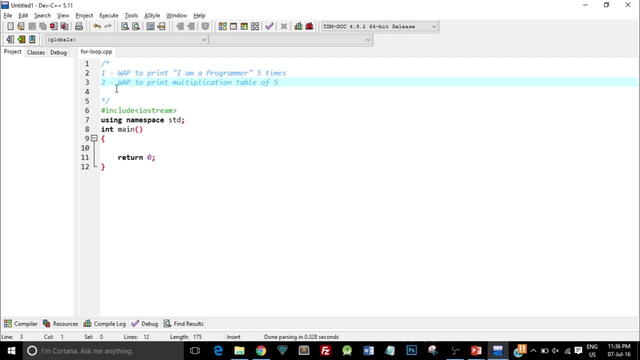 multiplication table of five. So before we start with the programming, let me tell you when we actually use a for loop. Now there are three different loop structures in C++, So it is for loop, while loop and do while loop. Now each of these structures are used. 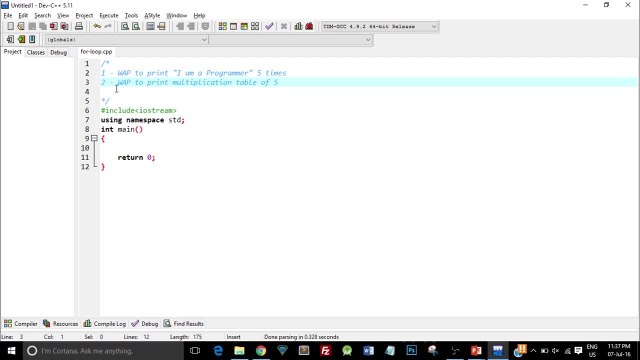 at different times depending upon the conditions. So when do we use this for loop? Now, for loop is used when we know how many times we are going to call the same thing again and again. So in the two questions, we know that the 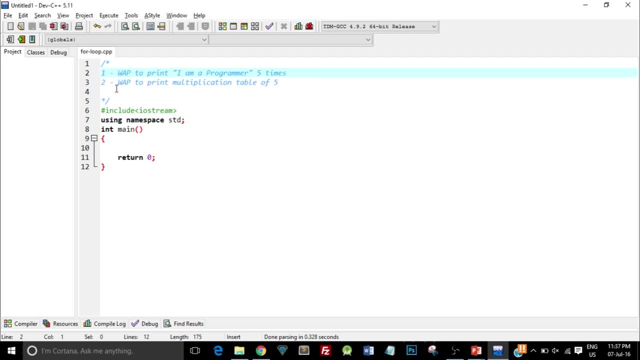 first question we have to print- I am a program of five times, That is, we know how many times we have to print it. And in the second question, we also know that we have to print the multiplication table of five, That is, we have to print 10 different numbers which are multiplicative. 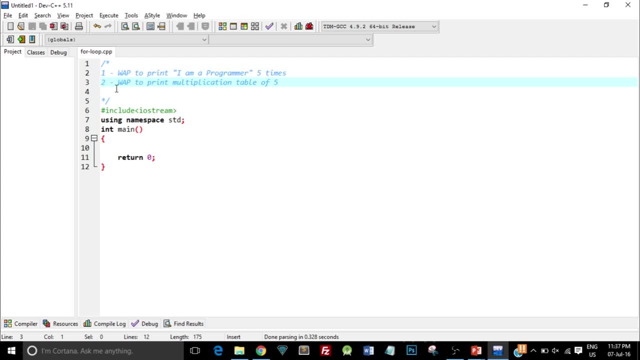 tables of five. So for loop is usually used when we actually know how many times we have to do something. So, with that being said, let's start with the programming. So here's the syntax for for loop: First type, the keyword for, then open and close parentheses or round. 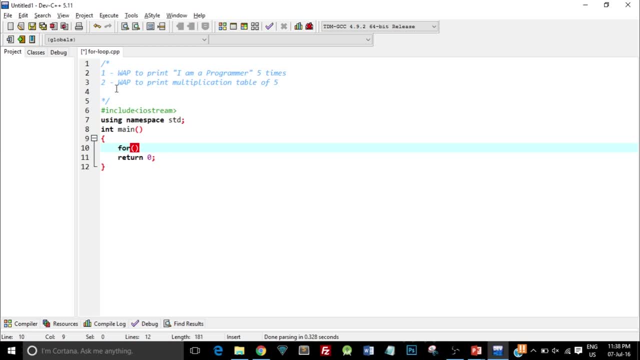 brackets. Now, inside these round brackets, there are three different parts. The first part is the initialization, The second part is the condition and the third part is the increment or decrement operator. So let me just type in and I'll explain you what is exactly happening. So 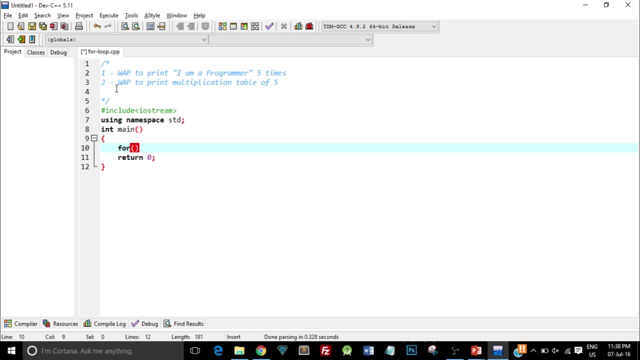 in the initialization I create an initialization variable, it- i equals to 1.. So this is the first part where I create a variable who's name is i and data type is integer, And I'm going to tell you the difference between this variable and this variable in general. So 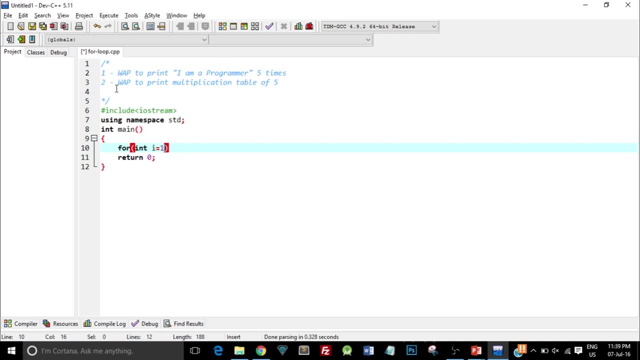 data type is integer and the value that it has at this moment is one. Then I type in a semicolon. So this is the first part. The second part is the condition. So I write I less than equal to five. So this condition means that this for loop should be executed. 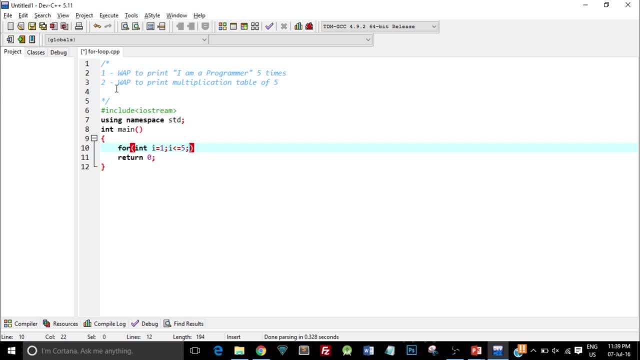 till I reaches five. Now again a semicolon. and here now I have to give the incremental factor, So I write I plus plus. So you know, this plus plus is an increment operator which will increase the value of I by one in every go. Then I open and close curly braces and 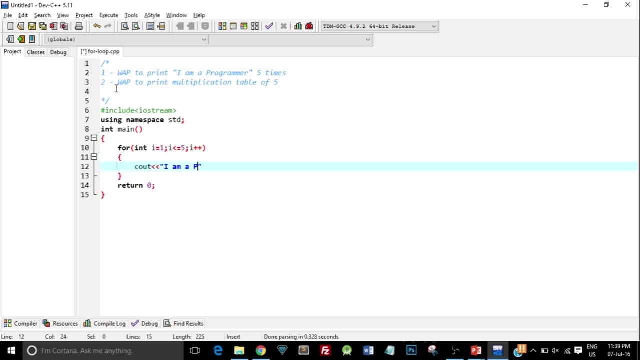 type in cout and I write: I am a programmer. Okay, so what will happen is when the program is executing, or when the program first executes. in the first go, the variable I value is one. It will check: is I less than equal to five? So, for the first time, I value is one. So, yes, I is less than. 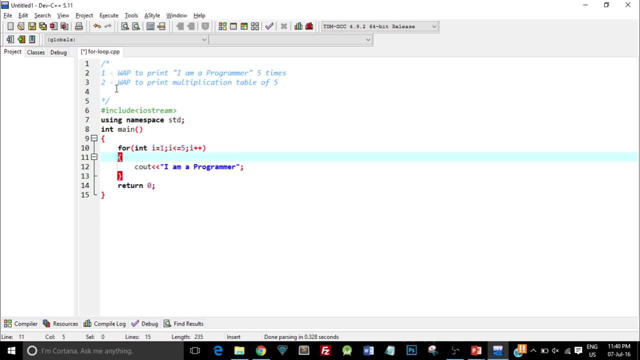 five. So this condition is true. So it will go inside this curly braces and print out: I am a programmer, So when we reach the end of this for loop, it will go ahead and increment the value of I, which is this incremental factor, and it will increment it by one. So now this: 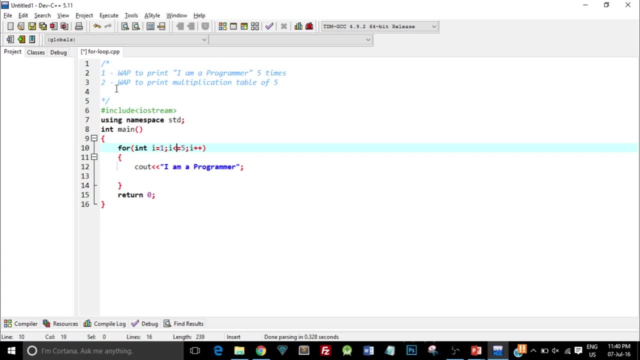 time the value of I is two, So it will again check: is two less than five? So as two is less than five, it will again go inside this loop and print I am a programmer again, and at the end it will again increment this I value to three. Now this will go on till I. 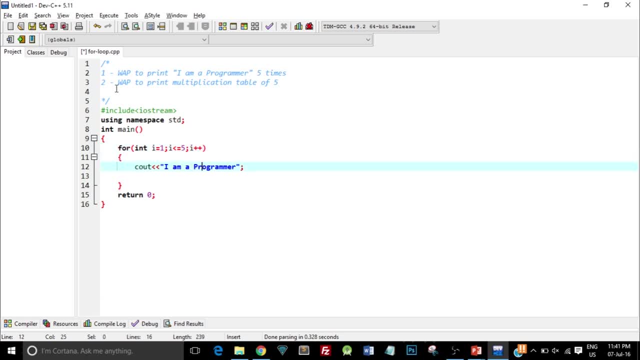 value reaches five, So five times it will print this I am a programmer sentence on the screen, and when the value of I is again incremented to six, it will check. here is I less than equal to five, Since I is six. so this statement becomes false or this condition become false. 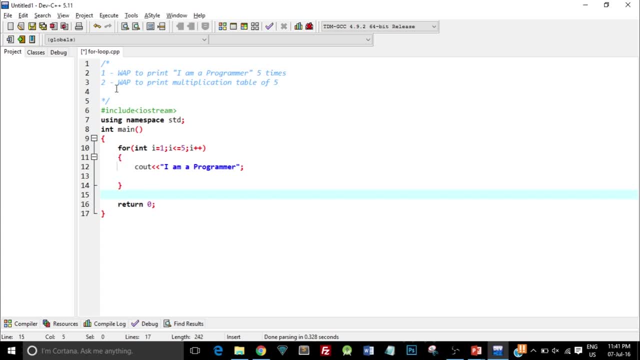 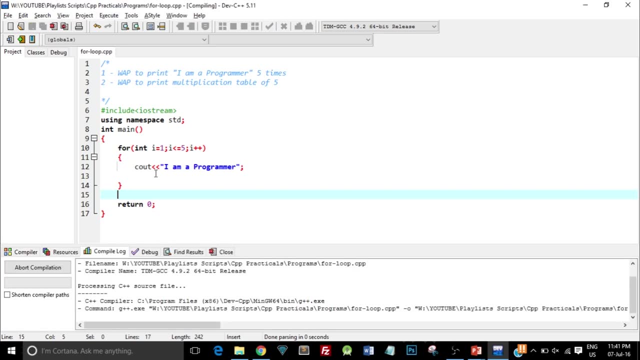 So it will exit out of this loop and it will stop this process. So I am a programmer, So process, so let me just go ahead and compile this and i click compile and run so it will directly run after compilation. okay, so you can see, i am a programmer. is printed five times, but then it is on. 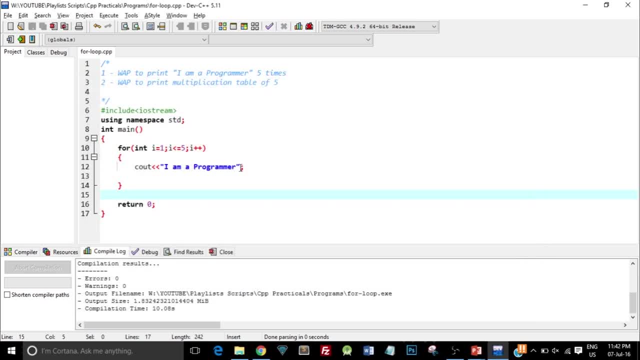 a single line. so let me just add one more thing to this output. i'll concatenate a end l which is sort of like an escape sequence, so every time you print it will go to the next line on the command prompt. so i'll just click compile and run and there you go. you can see it is printed for five. 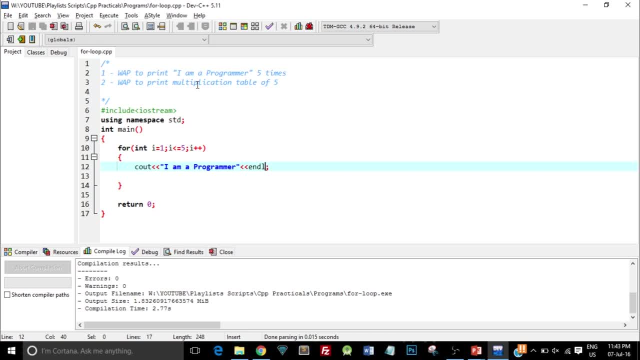 times. so let's see the second question, where, if we have to print multiplication table of five, so how do we do it? so here's what i'll do: i'll create a variable- int x is equal to 5, and then, at this line, i'll write 5. 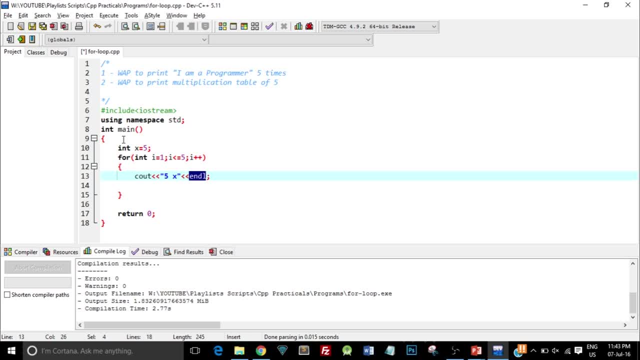 into, then i'll print the i value again, i'll concatenate a string and i'll write equal to and then i'll again print x, star i. and this has to happen at least 10 times because we need to print the entire multiplication table, starting from 1 to 10, so you might be confused. what exactly is happening? 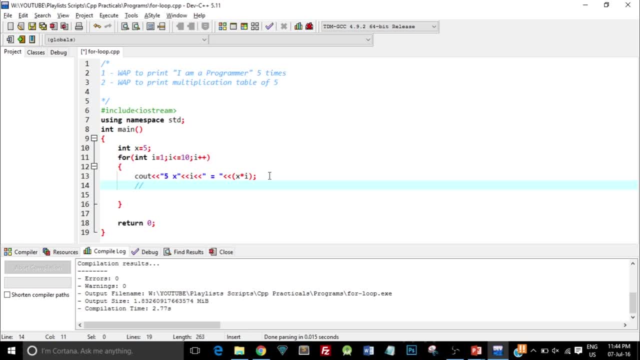 so here's what is happening. i'll write it in the comment in the first go. when i is equal to 1, this output would be 5. into this, i will be replaced by 1. then we have a equal to, which is printed as it is. 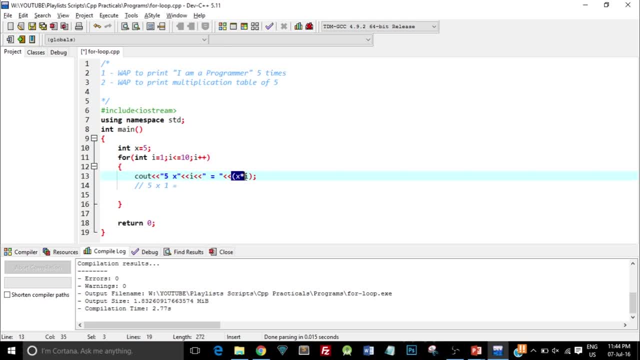 so it will come over here. and this is the expression where the x value is 5, which is- we have defined it at this line, and i value in this go is 1, so 5 into 1 would be 5. now for the second round. 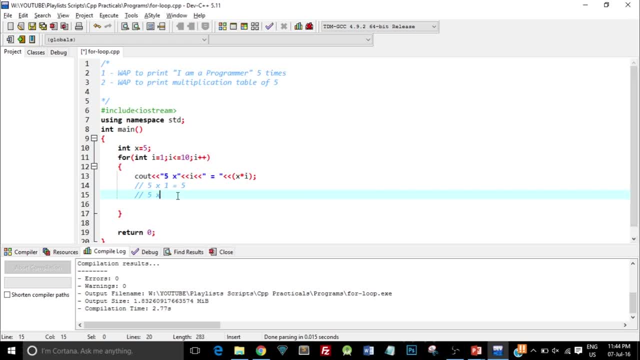 i value is incremented, so here it will be 5 into this time i is 2 and again this will remain 5, but this has incremented to 2, so 5 into 2 would be 10.. similarly, for 10 times we get the entire.